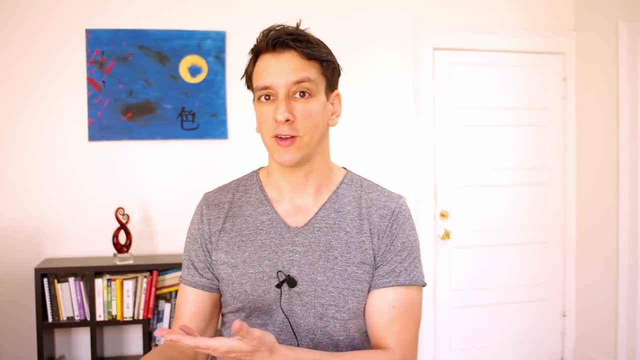 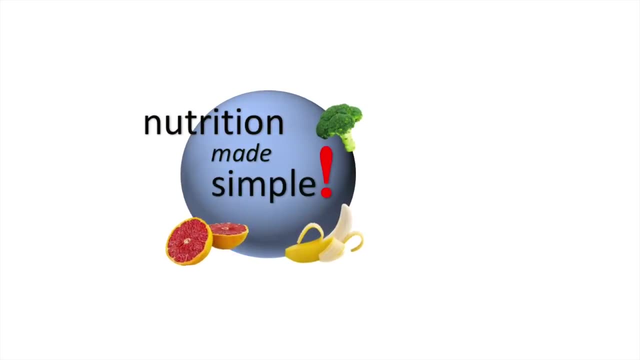 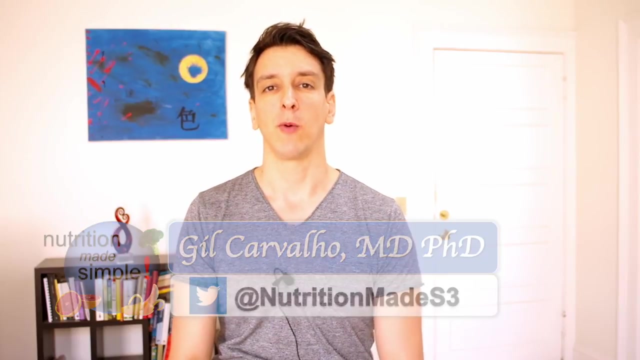 What is the best protein food source? Do we need meat for protein? Can we be healthy without it? Let's find out What's going on. this is Nutrition Made Simple. On this channel, we break down the science of food for your everyday use. If you're confused about what foods are healthy and which foods are not, then 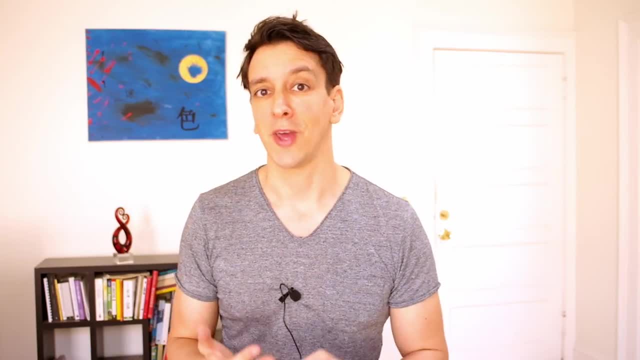 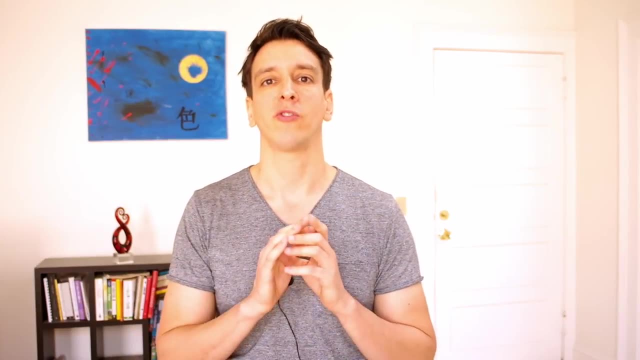 these videos are for you. Protein: We worry about getting more, about not getting enough, about getting the best Protein is an obsession, And yet we know almost nothing about it. So this is the first of a series of videos I'm going to make about protein. We're gonna cover 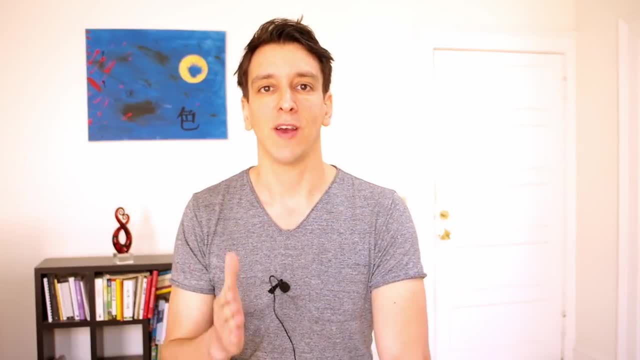 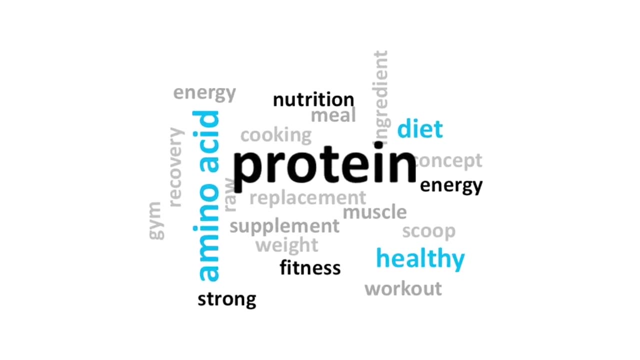 everything we need to know in order to have a healthy diet and never have to worry about protein ever again. Sound good. In this video, we're gonna focus on protein sources, which foods have it, which foods don't, and how much, Just to keep things interesting. quick question: 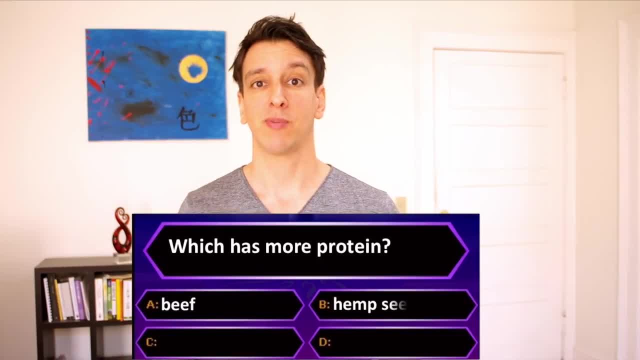 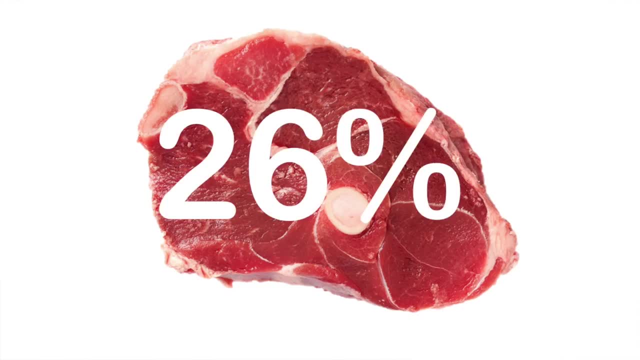 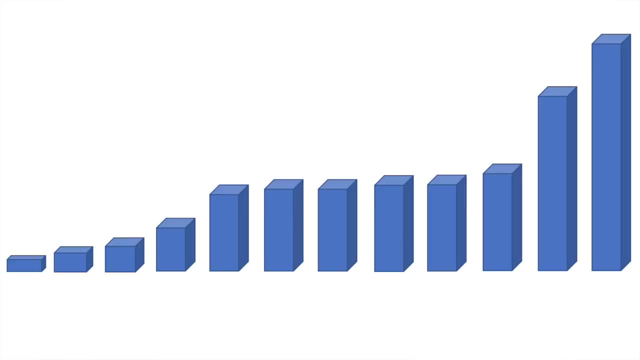 Which food has the most protein? Is it beef, hemp seeds, eggs or peanuts? Assuming same amount, say, one ounce of each Beef is about 26% protein, very substantial amount. So in a four ounce steak, about one ounce of that is protein. Now, if I showed you these 12 foods in order of the 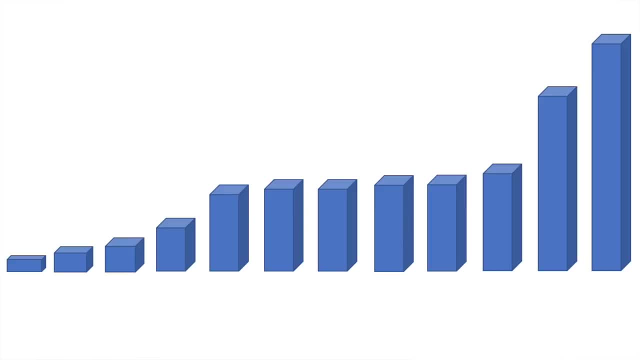 protein content from low to high. and asked you to guess which are animal and which are plant foods, Most people would guess something like this: Animal foods being the best sources and having the most protein, and plants with the least. And yet reality is a little different. 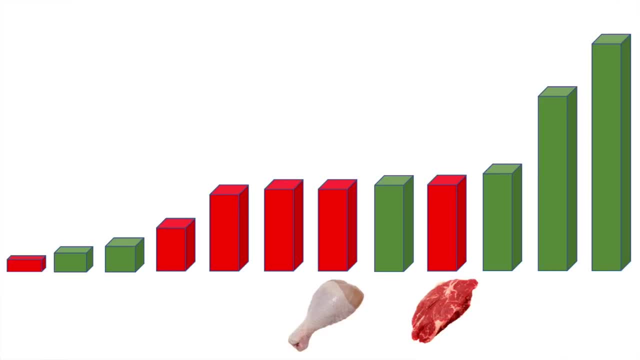 There's the beef with 26%. That's chicken, That's eggs and that to the left is milk. In the middle here we have peanuts: 26% protein, same as beef. To the right of beef We have hemp seeds with more than 30% protein and on the right we have seitan at 75%. 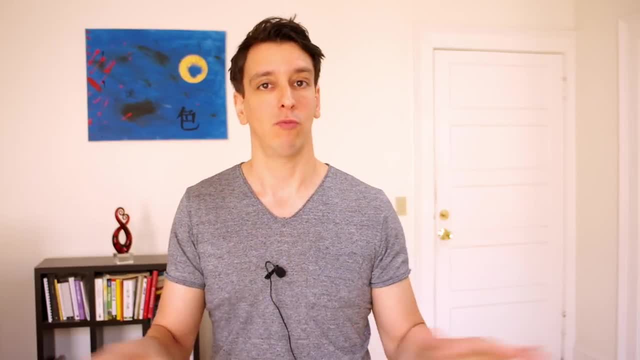 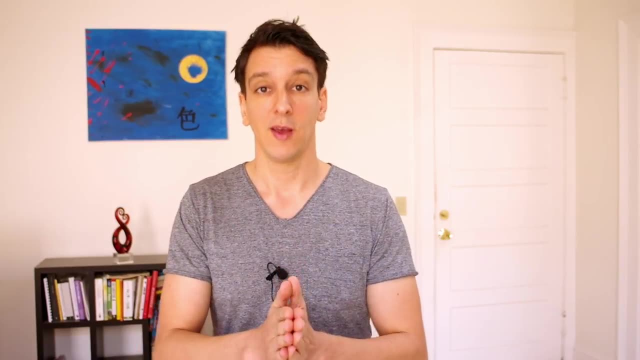 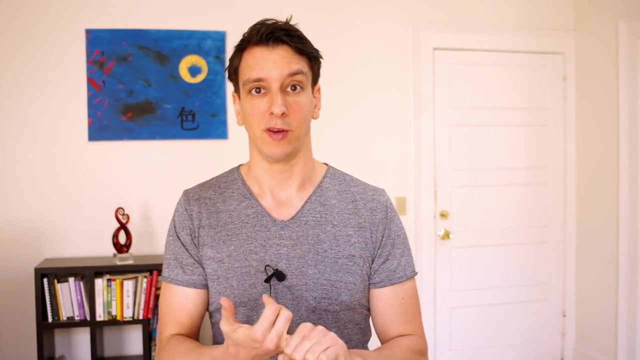 So am I saying that we should all start eating seitan three times a day? No, seitan wouldn't even be one of my top recommendations, since it's technically not a whole food. This is just to illustrate the point that protein is everywhere. All animal foods have protein and all plants have protein. The exact amount varies from food to food. 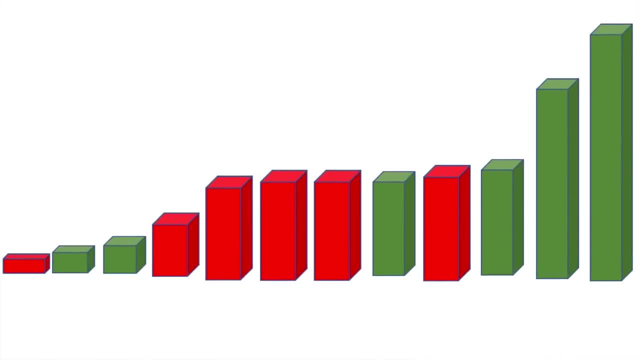 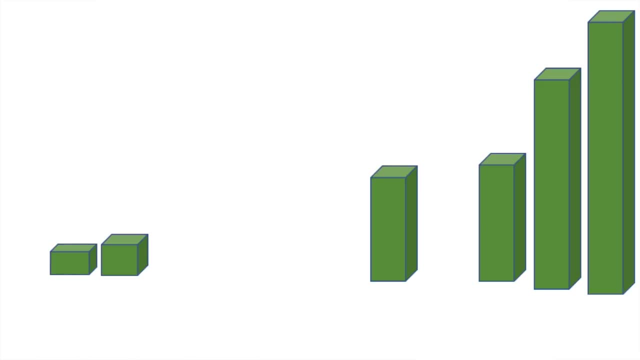 It varies among the animal foods and it varies among the plant foods, But whether you eat animal products or just a variety of plant foods, You're gonna get all the protein you need and in fact, studies have shown that vegetarians, pescetarians, vegans and omnivores all 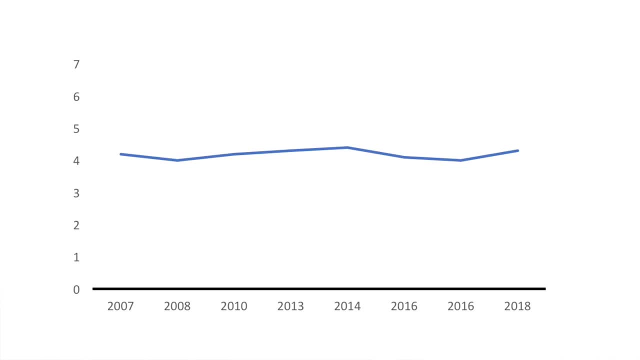 comfortably exceed the recommended amounts of protein. And, on a personal note, here are my protein levels from the last decade or so. The green shows the normal range. Before 2011, to the left of the red line. I was eating meat, dairy, etc. Like most people, and after that I made the changes to my diet and dropped all those foods. 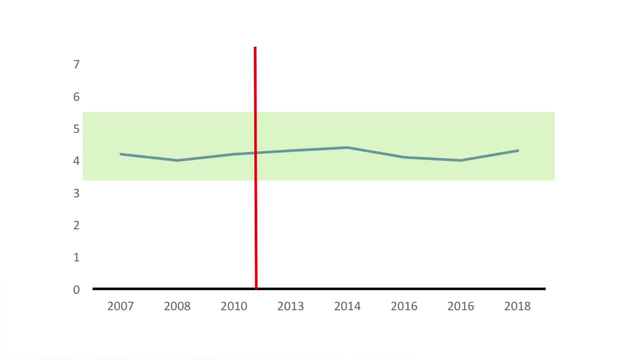 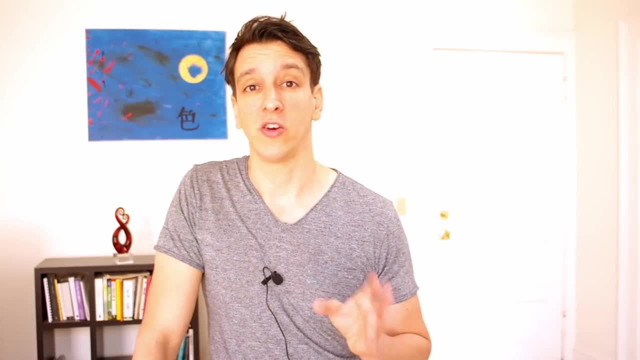 So you can see there's not much change and it's perfectly normal throughout, even though I haven't had a steak in seven years. No chicken, no dairy, and I eat fish and eggs less than once a year in average, So basically never. but I do eat a hundred grams of protein, give or take, every day. 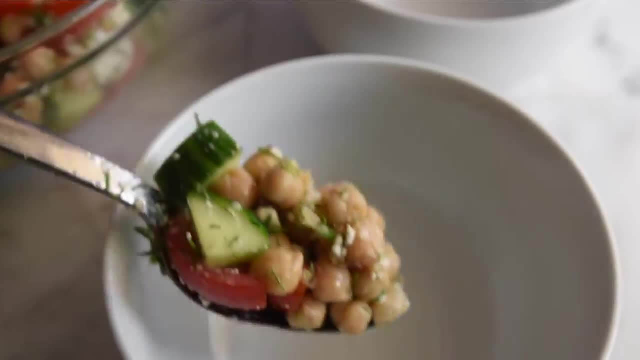 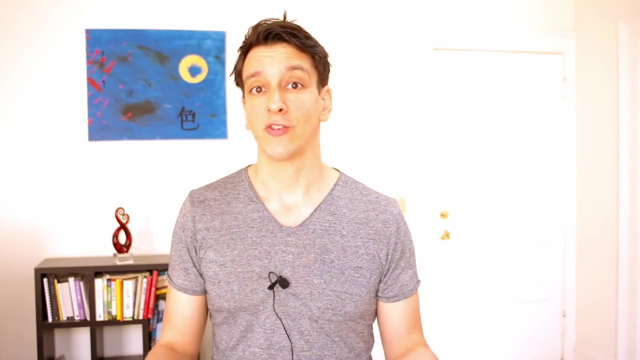 so the bottom line is we don't depend on animal products to get protein, and if we stop eating them all together, we're not gonna just keel over and die of malnutrition now. this reality is very surprising to many of us, myself included. 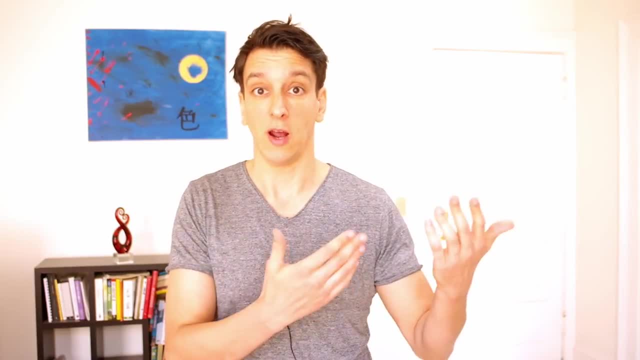 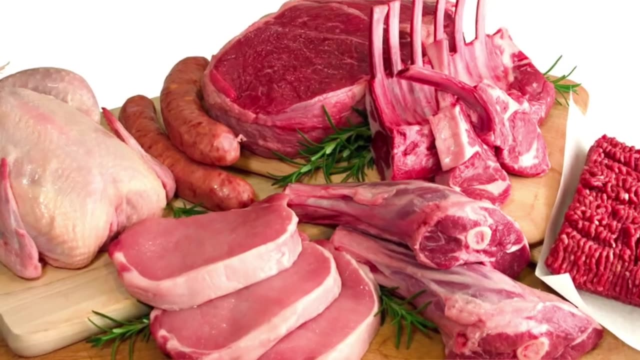 ten years ago. I would have been very surprised to find this information, as indeed I was when I found it, and the reason it's so surprising is that we are taught from a very early age that protein equals meat. this idea is all around us. chefs call meat the protein. 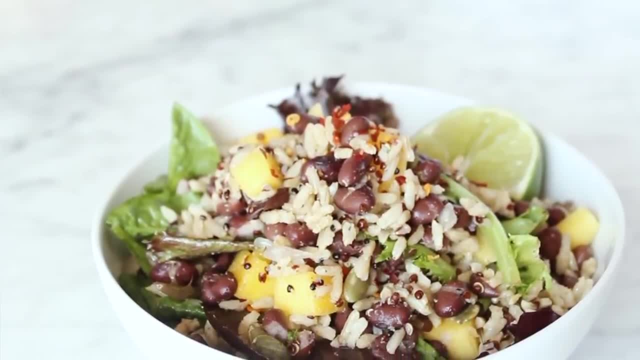 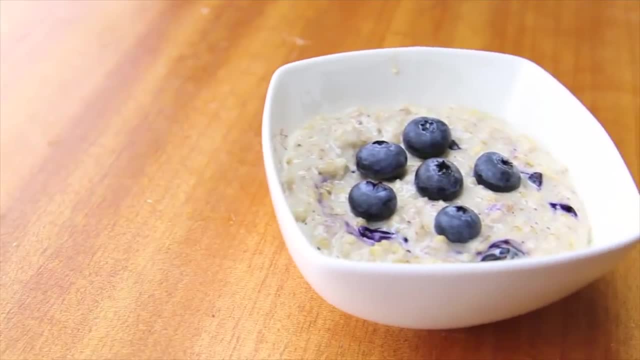 go to Chipotle, ask for rice and beans. the guy behind the counter will ask you: what about protein? your plate is already packed with it. here's another quick example to drive this point home. let's say I wake up and have a bowl of oatmeal and a peanut butter sandwich. a couple hours later I snack on some almonds. 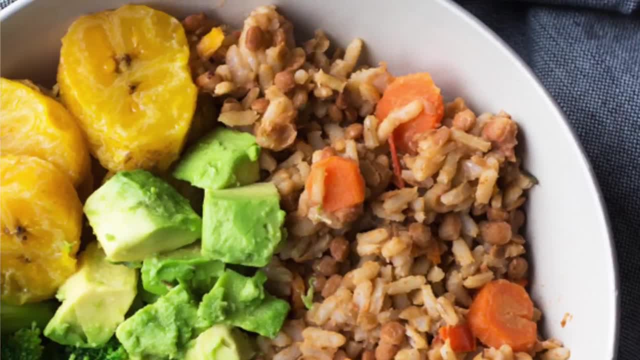 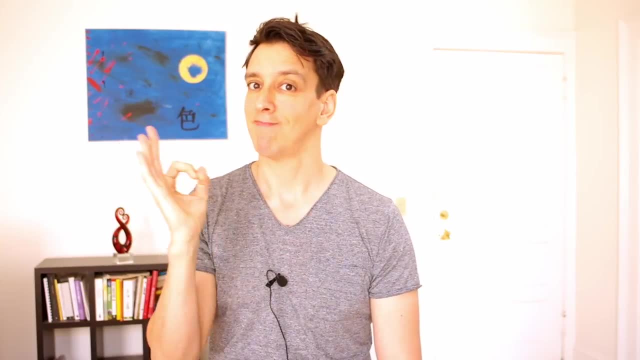 lunchtime: lentils, rice and some broccoli. one banana for dessert. how much more protein do you think I need over the rest of the day in order to meet my daily requirements? the answer is zero. the oatmeal peanut butter sandwich, the handful of almonds and that light lunch add up to 56 grams of protein. 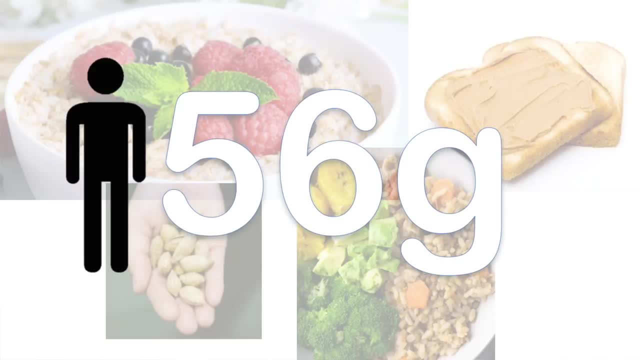 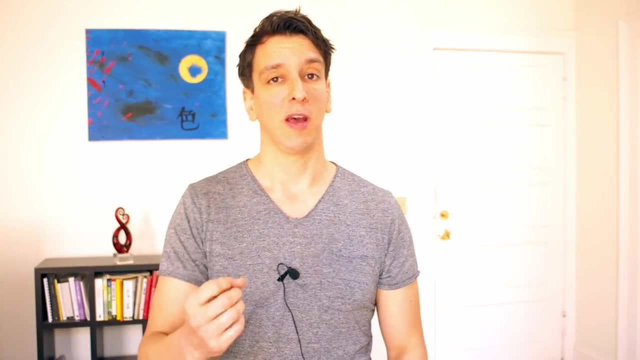 that's the daily requirement for the average man. if you're a woman, you've already exceeded your daily requirements by 10 grams, and it's just after lunchtime. now, if you're very active, you can have a bit more if you lift a lot of weights. you can have a bit more and in the example you still have dinner and whatever meals in between to go. so you're gonna eat more and that's fine. the example doesn't add up to enough calories for the day. plus, the protein doesn't get absorbed a hundred percent.